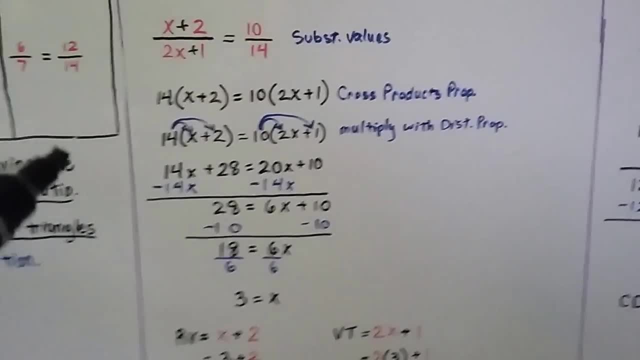 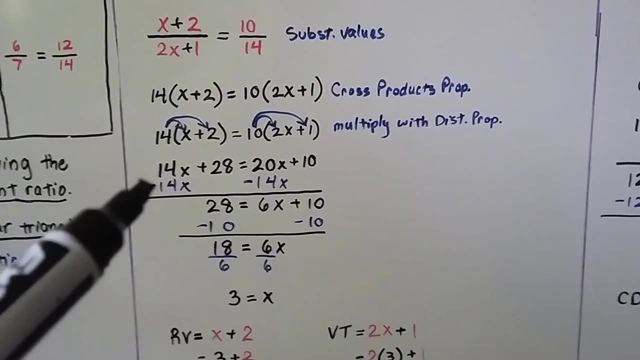 to 10 times 2X plus 2.. We can use the distributive property and we get 14X plus 28 is equal to 20X plus 10.. We subtract 14 from both sides and get 28 is equal to 6X plus 10.. We subtract this 10 and. 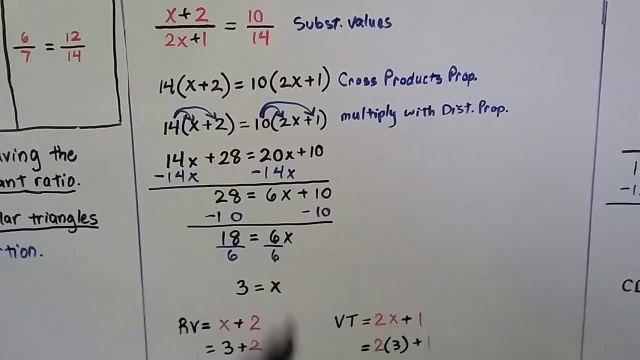 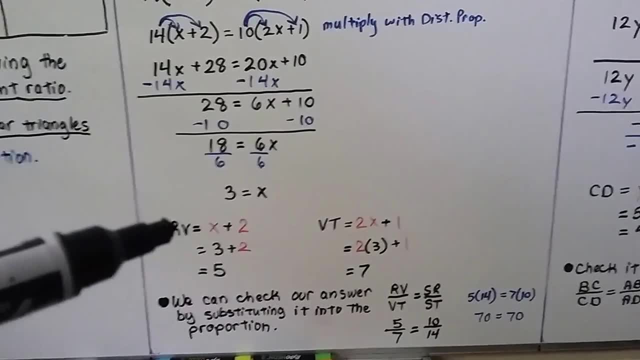 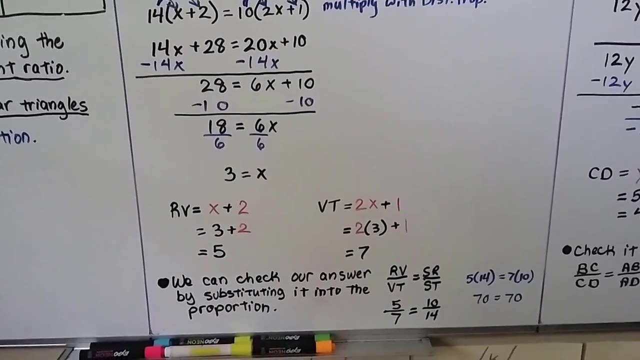 get: 18 is equal to 6X. We divide both sides by the coefficient 6 and find that 3 is equal to X. We substitute it into our expression and RV is equal to 5 and VT is equal to 7.. Now we can check our answer. by substituting it into the proportion, We would have a 5. 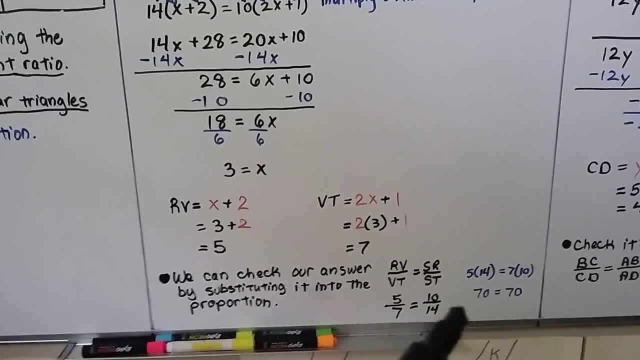 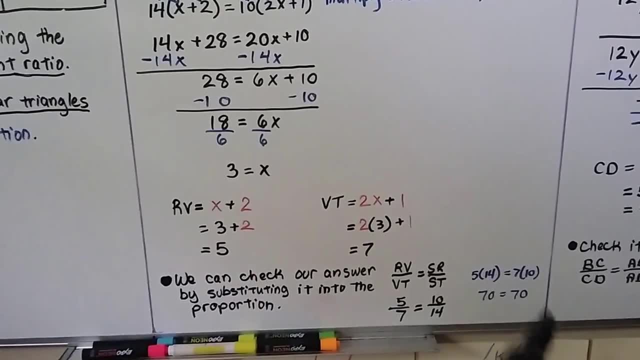 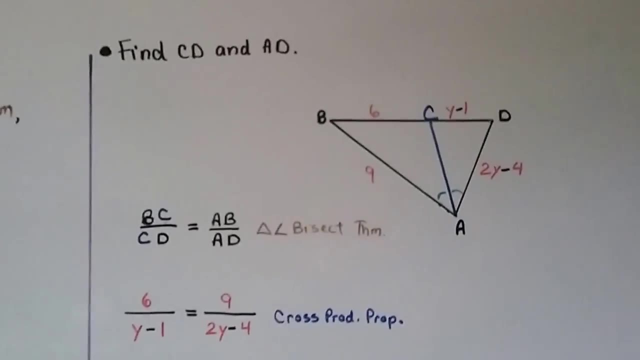 over a 7 is equal to a 10 over a 14. And that is proportional. We can even do cross-products and do: 5 times 14 is equal to 7 times 10, which is 70 equals 70.. Let's try one last one. We're going to find CD and AD. CD is Y minus 1 and AD is 2Y minus 4.. 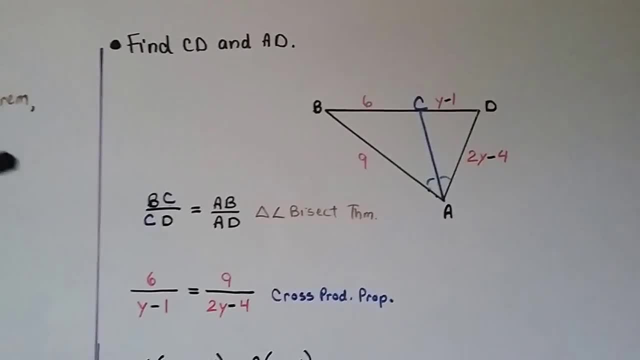 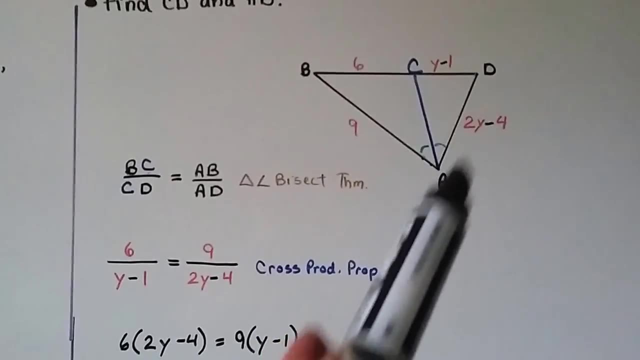 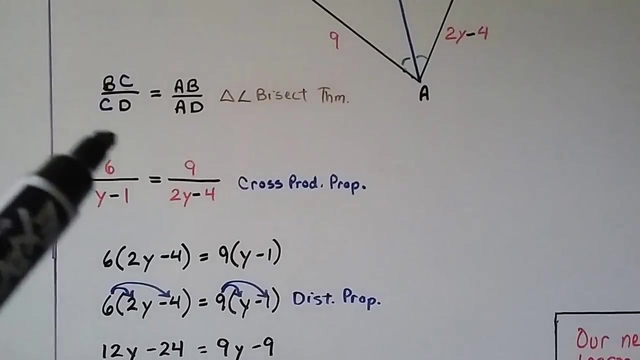 Using the triangle-angle bisector theorem, We write our proportion. We have BC over CD is equal to AB over AD. We substitute in the amounts the values and we can use cross products property. We have 6 times 2Y minus 4 is equal to 9 times Y. 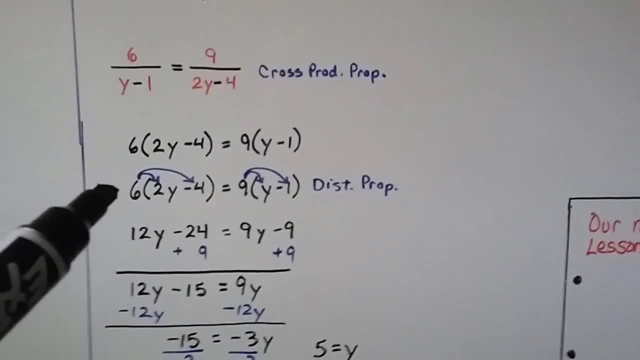 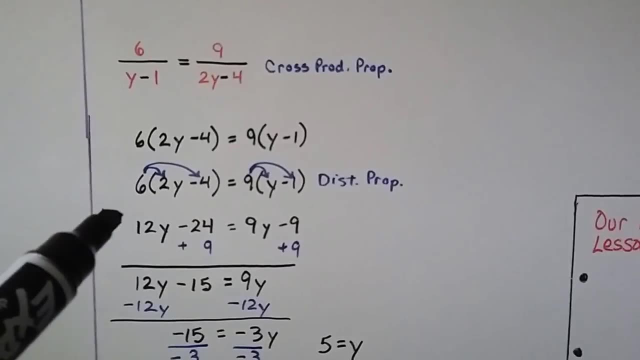 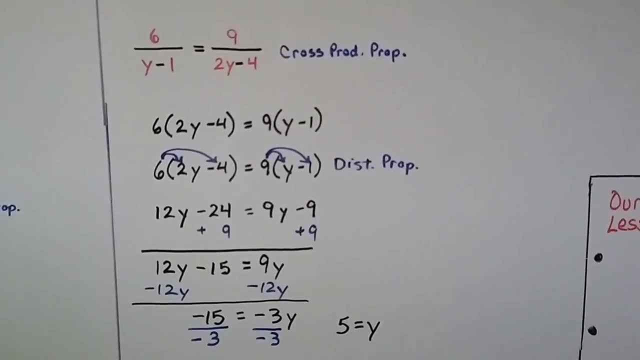 minus 1.. We use the distributive property and we've got 12Y minus 24 is equal to 9Y minus 9.. We add 9 to both sides and eliminate that, We've got 12Y minus 15 is equal to 9Y. We subtract the. 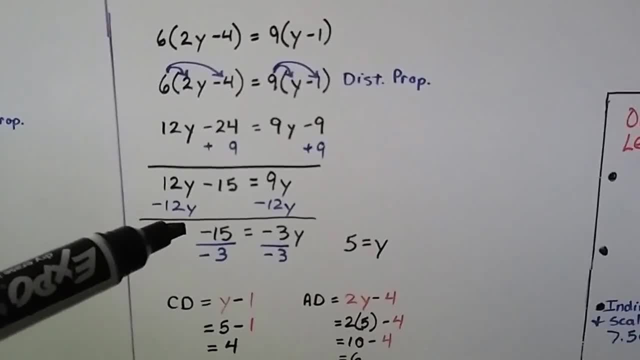 12Y from both sides and we have negative. 15 equals negative 3Y. We divide both sides by the coefficient negative 3, and we find that 5 is equal to 9Y. We subtract the 12Y from both sides. 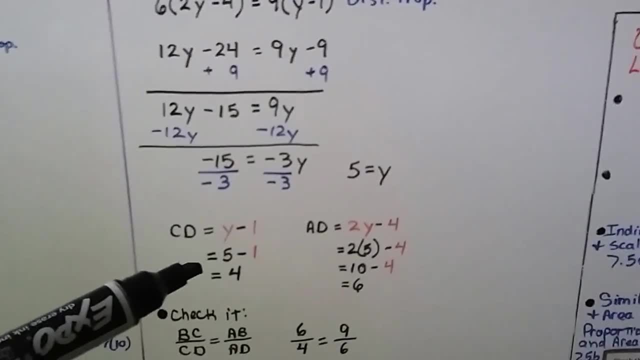 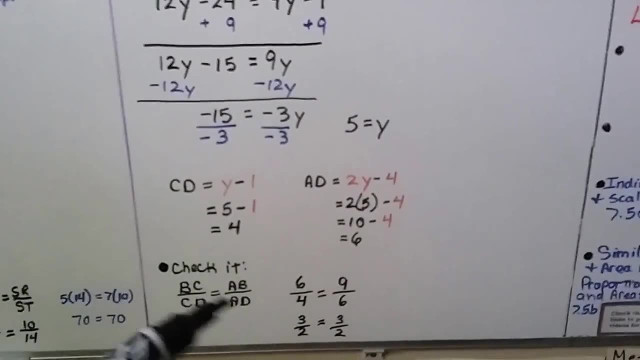 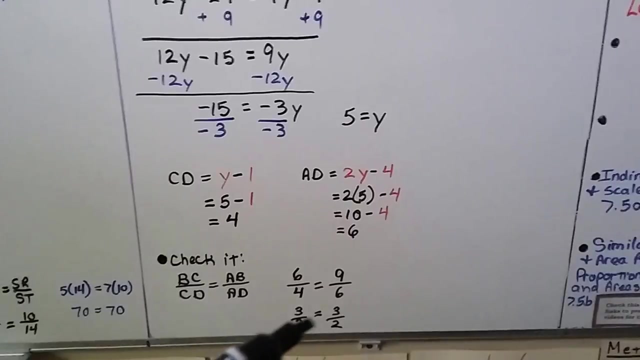 equal to Y. Now we can substitute that in to the expressions and we get: CD is equal to 4, and AD is equal to 6.. We can check it by putting it into our proportion and we have: 6 fourths is equal to 9. 6,, which means 3 halves, is equal to 3 halves. And yes, that worked All right.